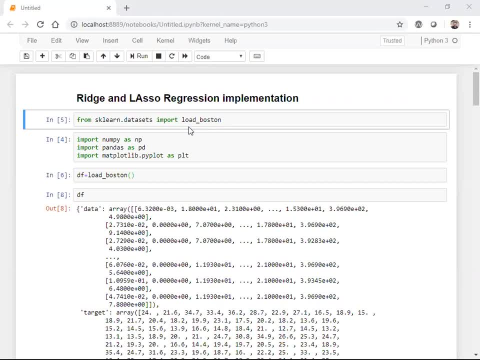 This load underscore. Boston basically has a data where we need to predict the price of the house based on various features. We'll try to discuss about that, which all are the other features that are actually required. So first of all I'm going to load this particular Boston library. 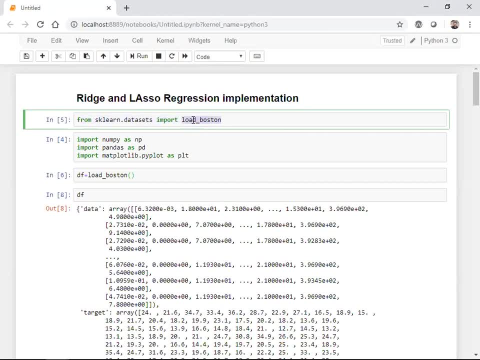 Already, the data set is present inside this particular library. We'll initialize it and we'll just load the data. After that, we are going to import libraries like NumPy Pandas and Matplotlib, which is pretty much important because I'm going to do some of the plottings. 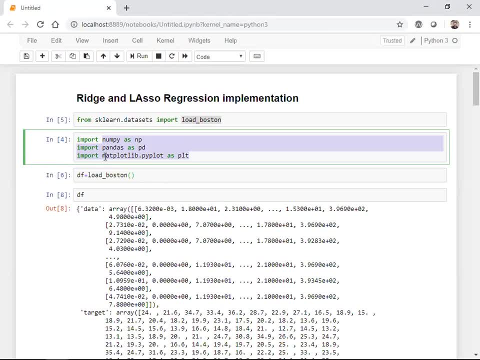 So there, this is actually required. And in this particular video, what we'll do? first of all, we'll try to implement this with the help of linear regression. Then we'll go and implement ridge and then lasso regression, And you'll be seeing that there will be a mean squared error. 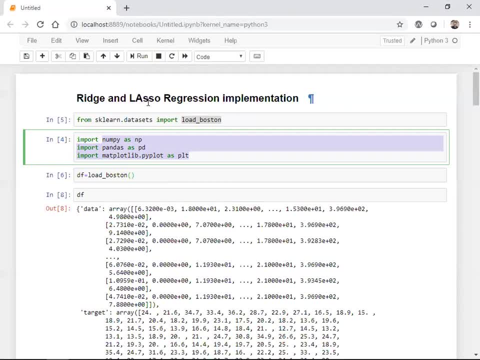 The error will be reducing as we go ahead with ridge and lasso regression. And you know why it happens, because I've already explained in the theoretical explanation that I put up yesterday. If you have not seen that particular video, I'll give the link in the description. 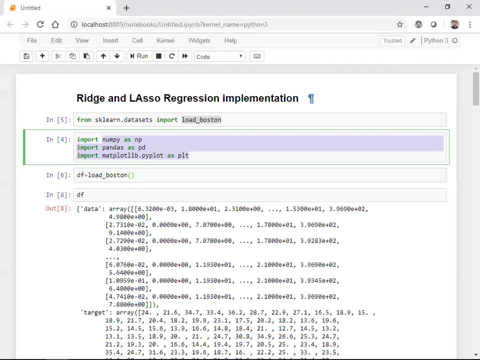 You can go and actually watch The complete Theoretical understanding of ridge and lasso regression. The tutorial is just before this particular tutorial, right? So now I'm going to initialize Lord underscore Boston, Lord underscore Boston. So by default we'll be getting this whole data. 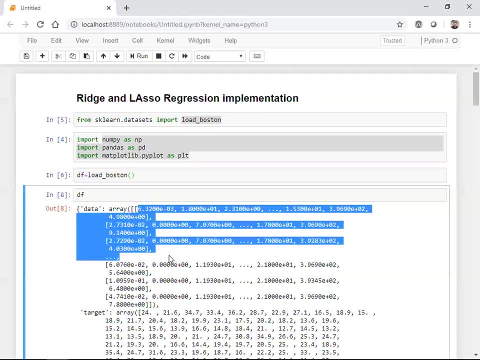 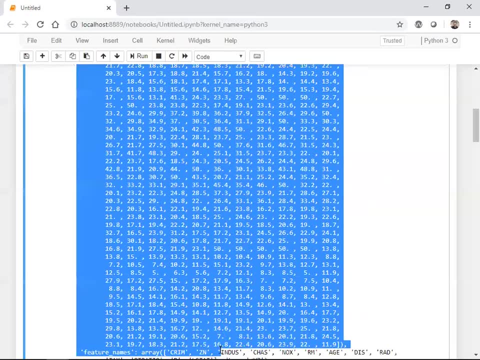 This data basically indicates what are the values based on the number of features. So this will be the array format. These are my targets, So this target is basically my price of the house. OK, so these are all my price of the house. 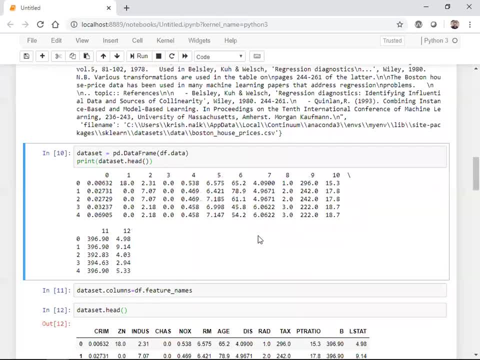 These are my feature names, So I'm just basically showing you everything. Now, the first thing is that we will try to convert that into a data frame. So I'm going to take the F dot data, I'm going to convert that into a data frame and store it in a data set. 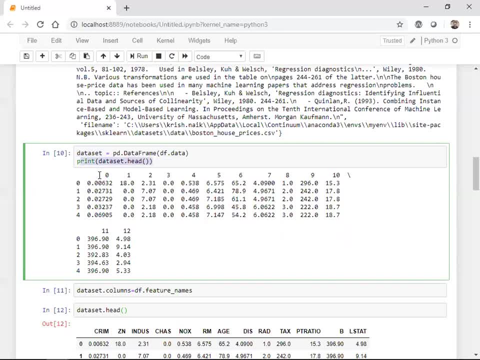 After I do this, I'm going to print the data set dot head. Now, here you can see that these are all my independent features, Guys, since I've just taken the data part right. my dependent feature is basically the target variable. 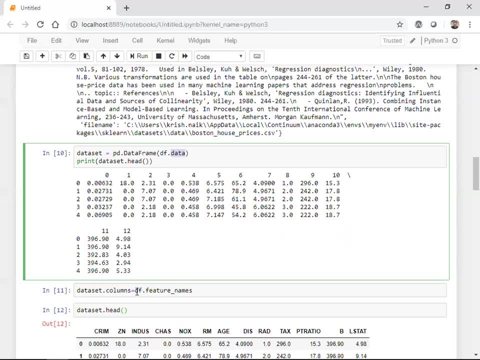 OK, so that I'll be loading later on. Then what I do is that I'm going to use the F dot feature names and I'm going to assign to the all this particular data set columns, Right. So here you can see that. 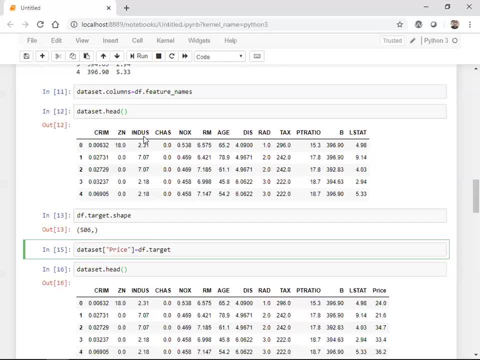 After I execute this, these are my columns Here. I am That in this class. you know X, R, M, H, D, I, S, R, X. If you want to understand all this particular feature, you can just go and have a look at that load on the school Boston library. 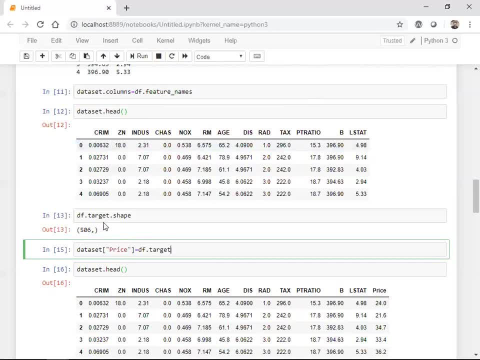 You'll be able to understand everything. Now, the next thing is my dependent feature. for my dependent feature, I usually take it from the target dot sheet. If I do that, if they are, they are total five zero six rows. So I'm able to see over here and what I'm going to do is that in this particular data set I'm going to create, 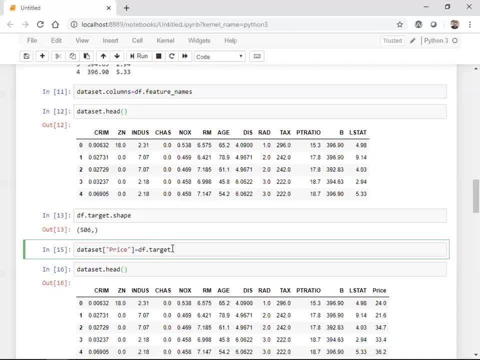 A new column called a price and there I'm going to put this target variable. So this is the code that actually does that data set of price is going to be a target. Pretty much easy till now. Now, when I go and see my data set dot head here, here is the output that you can basically see: the top five records. 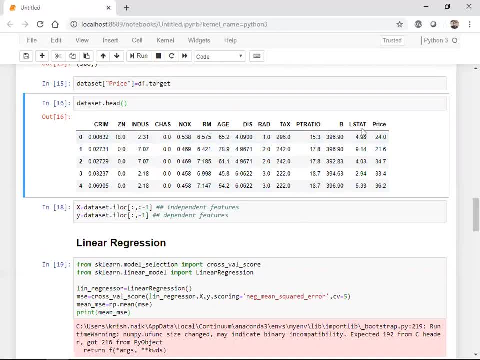 You have your dependent features, price and all your independent features over here Right now. the next thing that we do is that divide this into independent and dependent feature. OK, now let us go ahead and try to implement a linear regression. So linear regression. 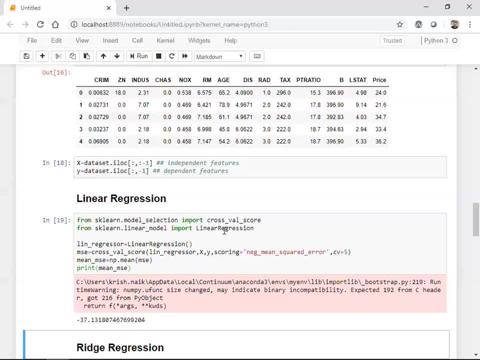 I hope everybody knows how to implement it. So first of all, I'm going to import linear regression from a skill under linear model. I'm going to import this linear regression and then I'm going to use cross valve score. Cross valve score is basically used to do cross validation. 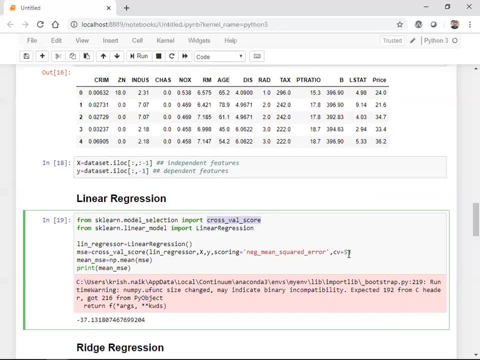 And here I'm going to perform five cross validation. That basically means five experiments inside my cross valve score. I'm going to put my linear regression object, which I've initialized over here, my X and Y value, which is my independent and dependent feature. 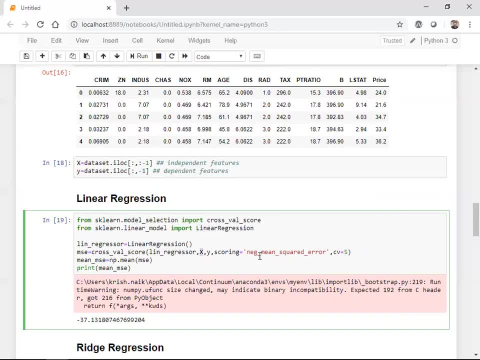 And And scoring that we are going to use over here is a negative. And there's four mean and there's four square and there's four error. This is basically mean and there's four square, There's four error. Usually, whatever the mean square error we get, we are going to put it as a negative value. 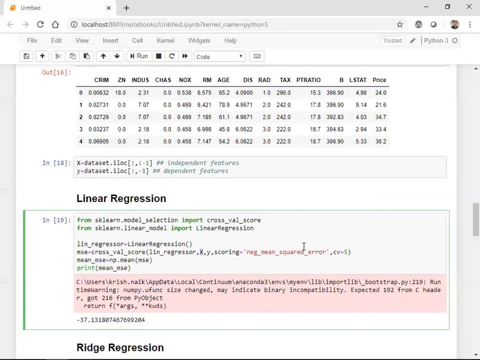 And remember, this value should be very much zero to zero. The more it is nearer to the zero, the more the model performs well. OK, So when I do it mean so, based on this particular five experiments, or five cross validation, I'm going to get five values in the form of bliss. 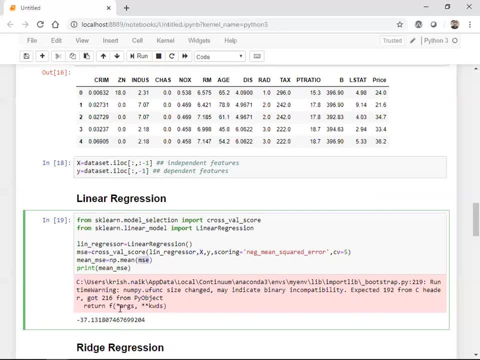 Then I'm going to do: and people mean, of MSE. That is a mean square error. And finally, we can see that as soon as I execute this, I'm getting a mean squared error of minus 37.13.. Now, since I'm using negation, 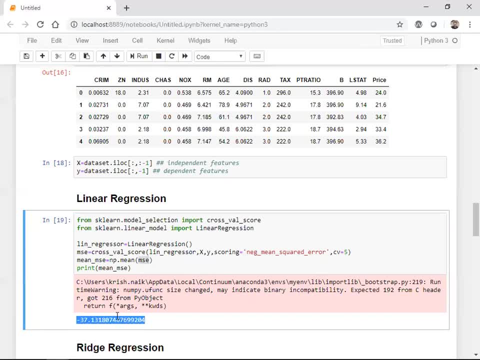 so it is giving us a minus 37 and this value should be nearer to zero. The more it is nearer to zero, the more the model is actually giving an accurate result. But again, you should also understand it may also lead to overfitting. 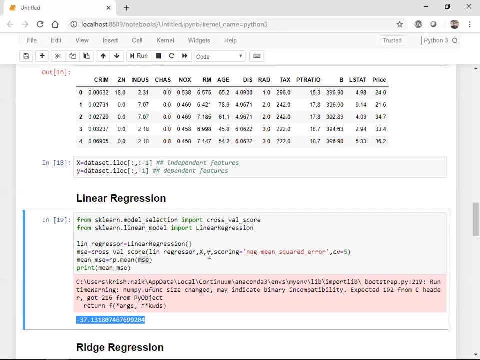 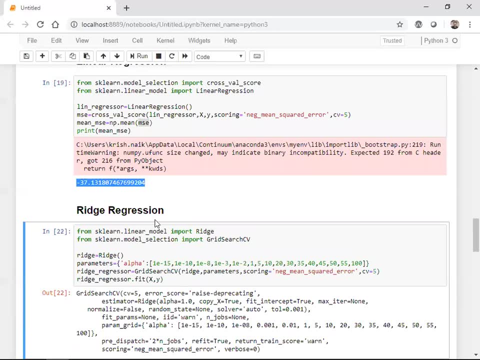 But let us go and understand how we can implement the same thing, or we can create a model with the help of ridge and lasso regression. So in the next slide I've actually introduced ridge regression and I told you that guys, in ridge regression also. 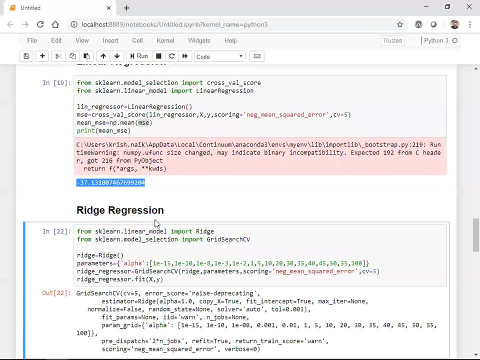 we need to find out a value which is called as lambda, And that lambda is basically also found out through cross validation, And for that we are going to use grid source CV. So what I'm going to do? first of all, I'm going to initialize or import linear model. 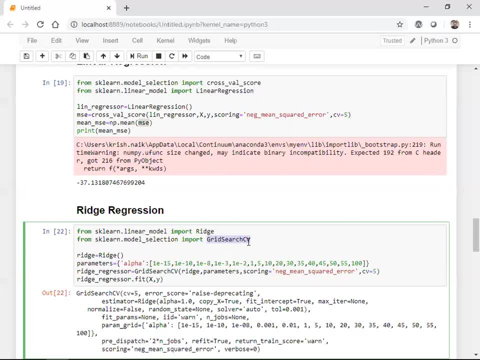 I'm going to import the ridge, Then after that I'm going to import grid source CV, And it is again present in the same library: linear underscore model and model underscore selection. Then what I'm going to do is that I'm going to initialize this ridge. 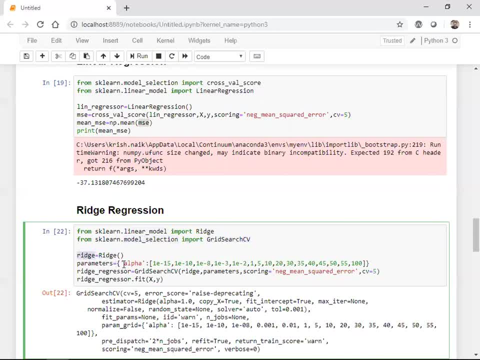 object. okay, Then over here you can see that this is the parameter that I actually require inside my ridge. Now I'm going to actually perform grid source CV, So usually what happens is that I will provide various different values for alpha. Now, the first value that you see over here: 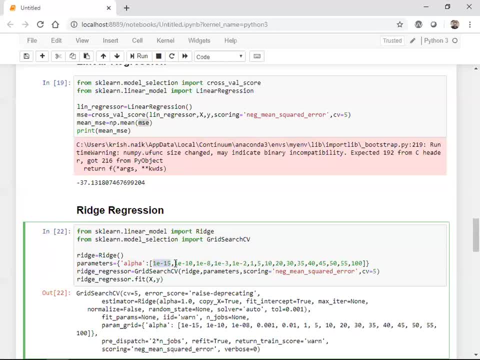 is nothing but 10 raised to minus 15.. The second value is 10 raised to minus 10,, similarly, 10 raised to minus eight. minus three minus two, one, five, 10,, 20,, 30,, 35,, 40,, 45 till 100, okay. 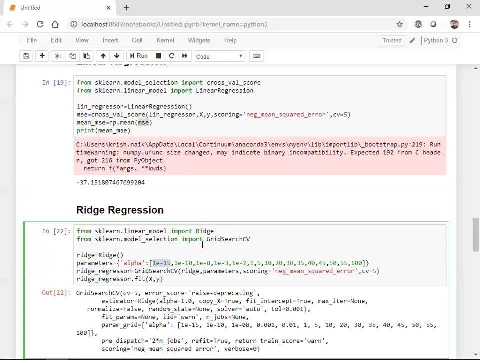 And remember, the alpha value should always be greater than 10.. So, remember, the alpha value should always be greater than 10.. So remember, the alpha value should always be greater than 10, and it can be any infinite number, okay. Any finite number, sorry. 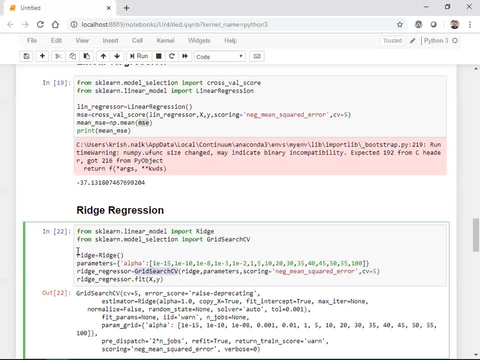 Then what I'm going to do is that I'm going to initialize grid source CV. The first parameter will be my ridge object, Then the parameters that I'm going to select, because, with the help of this grid source CV, I'll be able to find out which alpha value 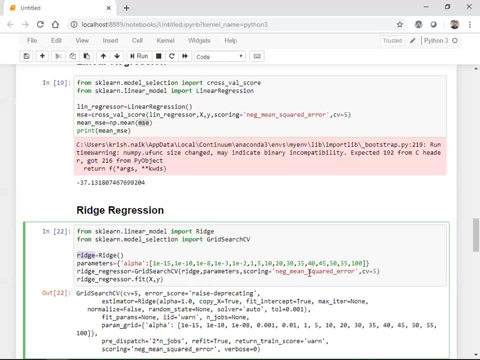 suits for this particular problem statement. And the scoring is nothing but again, negation, mean underscore, squared underscore, error because we need to compare with the linear regression right, And here I'm also taking the cross-validation of spine. So as soon as I execute this, 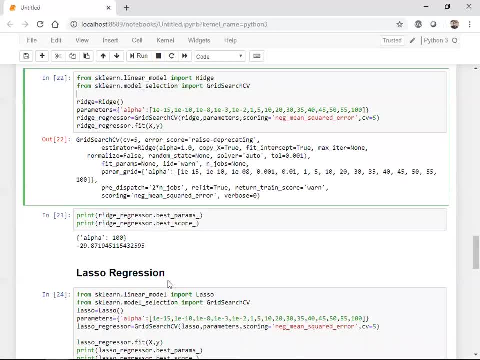 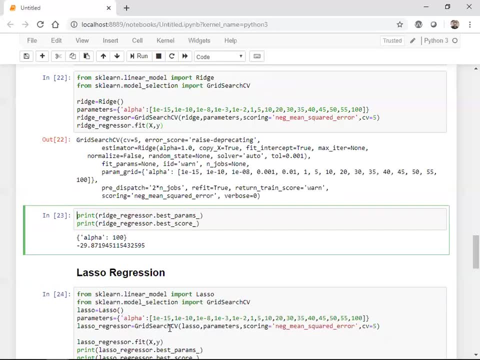 then I have to do fit X and Y. Now the next thing is that I want to find out which is what will be my minimum squared error. So for finding out that I need to print best underscore score, This best underscore score will actually give you. 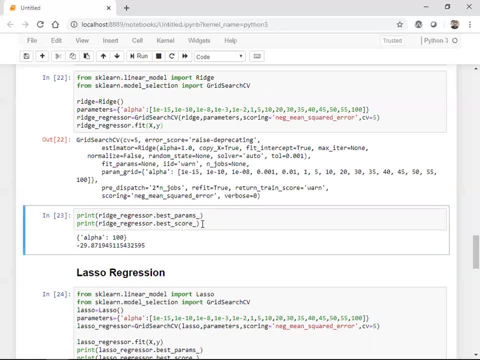 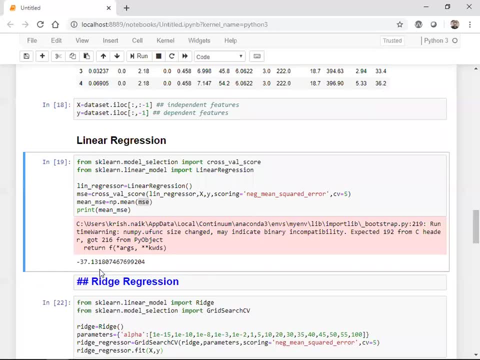 the mean squared error. okay, So ridge underscore regression dot. best underscore score is the property name. Now here you can see that I'm getting minus 29,. okay, So it is quite good than minus 37,, because minus 29 is more near to zero, right. 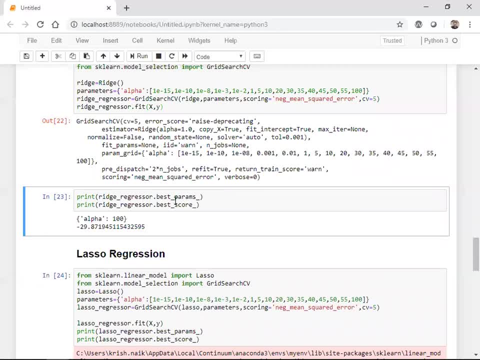 Then this best parameter actually help you to find out which lambda value was the suitable or which lambda was suitable enough. So here it has been selected as 100.. So you can see that one of the value was 100 over here and that has got selected. 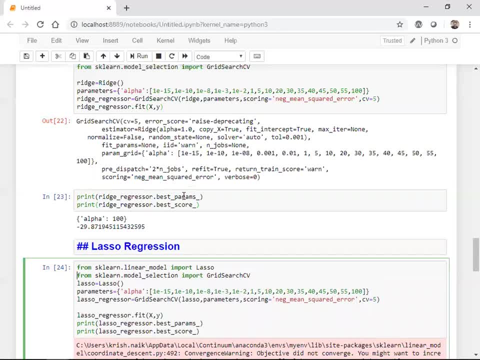 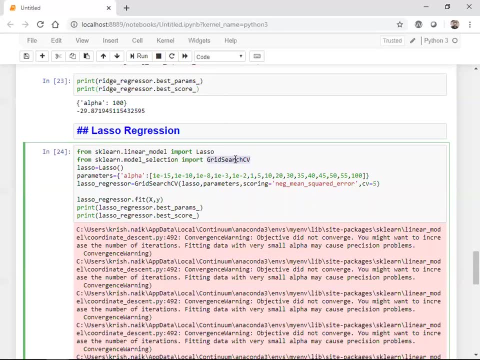 Similarly, if we go and perform with the help of lasso regression, in lasso regression also, we do the same thing. We actually import. let me just show you: we actually import lasso, then we import grid-srcv, then again we initialize lasso. 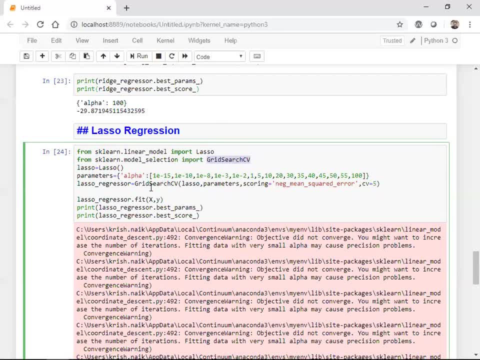 provides different kind of alpha, that is, lambda parameters. with the grid-hub-cv, grid-hub-cv, grid-srcv, we use the lasso object and then we are providing the parameters with the same scoring and cross-validation. 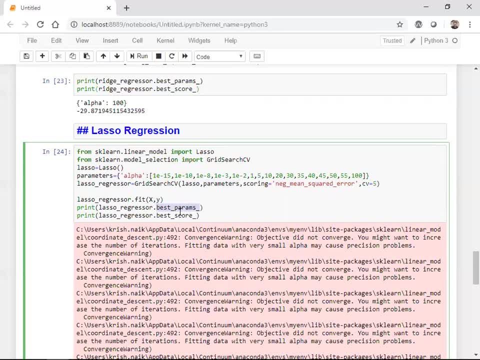 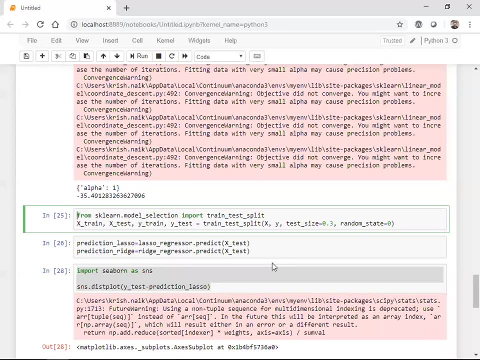 When we do fit x and y and we find out best underscore params and best underscore once we execute it, we'll get some kind of warnings. You can ignore this warning for now, guys. Then the alpha value that is selected is one. 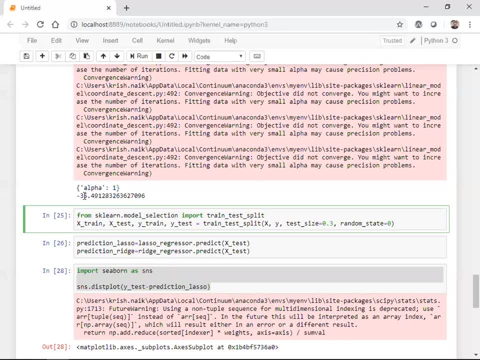 and the minimum squared error is minus 35, which is pretty much good than linear regression. but understand this: minus 35 is considered and lasso regression. you know that what it does is that for some of the features it will completely ignore. 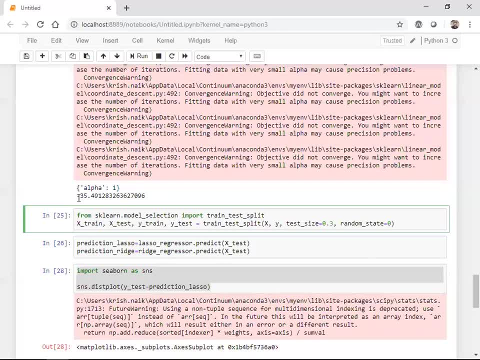 because, remember, if from my theoretical video that you have understood in lasso regression, what we do is that we just not minimize the minimum squared error plus lambda multiplied by magnitude of slope, not slope squared, okay. So because of that, 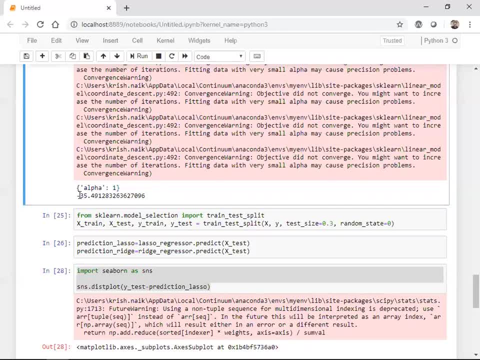 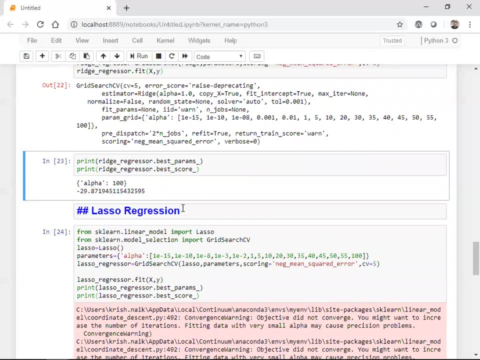 this particular value looks like a more generalized model. but just don't consider that, since we are getting in the, you know, in the ridge as minus 29,. ridge is better than lasso. Lasso performs well when you have many number of features. 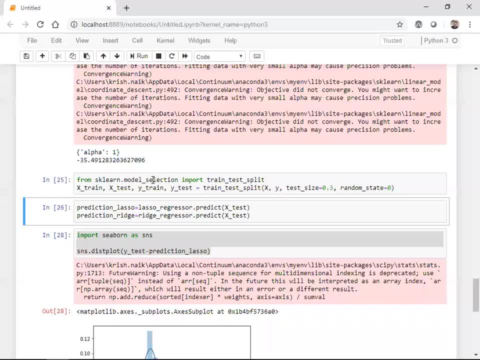 okay, So here it is. Then what I do is that after that I do test split, I want to verify it for X underscore test, and so this is my prediction: underscore lasso: where I'm using lasso underscore regression: dot predict. 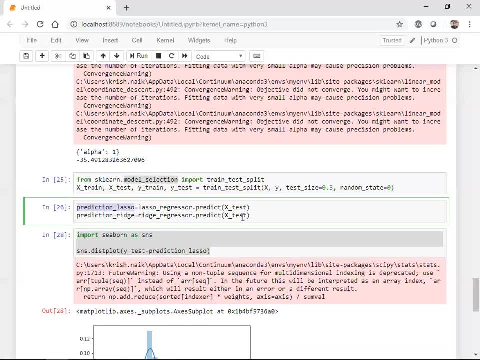 and prediction underscore ridge where I'm using ridge regressor dot predict of X test. So both the output I've got over here. what I can do is that finally I can plot it. I'll be using a distance plot and this plot.